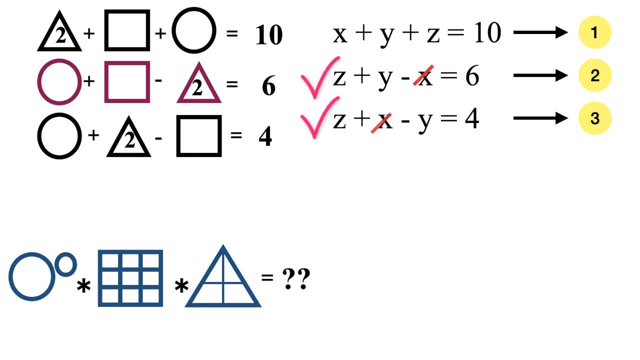 now solve equations 2 and 3. cancel y and x, equation becomes 2. z equals 10, thus z is equal to 5. thus value of circle is 5. now substitute the value of x and z in equation 1. after solving equation 1, equation becomes y plus. 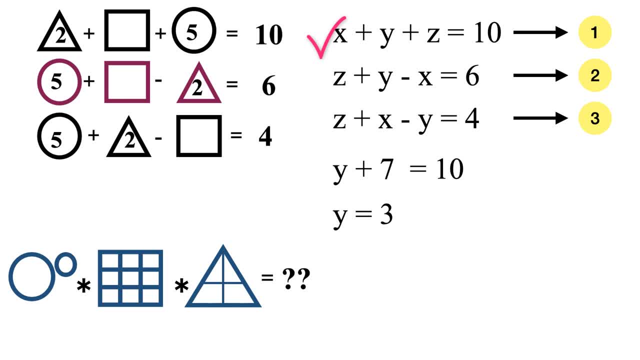 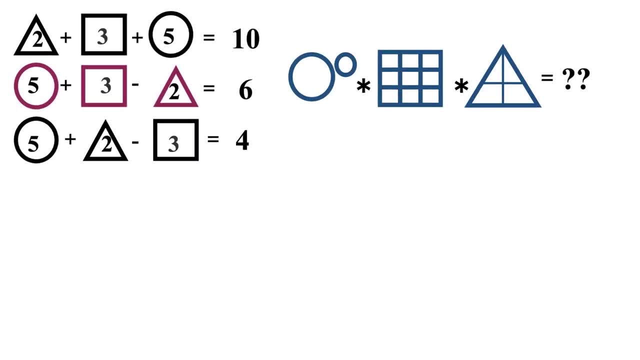 7 equals 10 after solving, the value of y is 3. thus value of square is 3. now we know the value of circle, triangle and square. value of triangle is 2, value of square is 3 and value of circle is 5. let's get into the most interesting part of the problem now, the most difficult part of the problem. 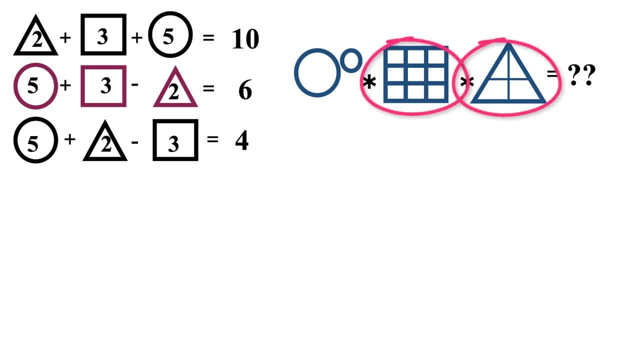 lies in finding total values of y and z number of squares and triangles. in second and third figure of the last row, number of circles is intuitive. that is number of circles as clearly visible. it is 2. there is a shortcut to find the number of squares and triangles, which we have already published. check the description section. 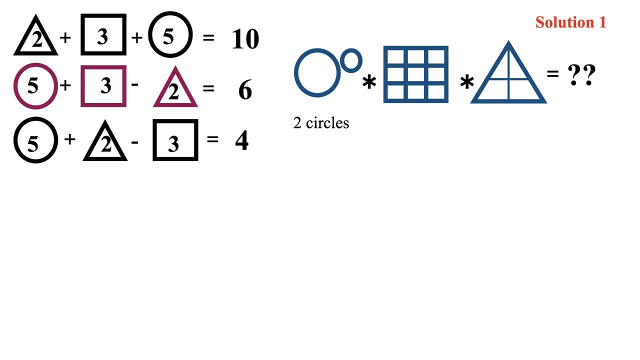 to know more details. in the first look, most of the people thinks that the number of squares in second figure is 9, but if you closely look there are 1 cross 1, 2 cross 2 and 3 cross 3 squares, after counting number of squares and triangles. in second and third figure of the last row number of squares. 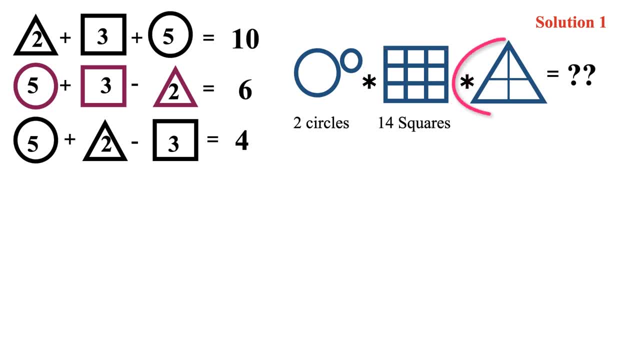 is 14. similarly, number of triangles in third figure is 6. as i have already mentioned, there are two solutions to this problem. let's check the first solution. if you interpret the first figure as just circles, then there are 2 circles and 14 squares and 6 triangles. since we already have the 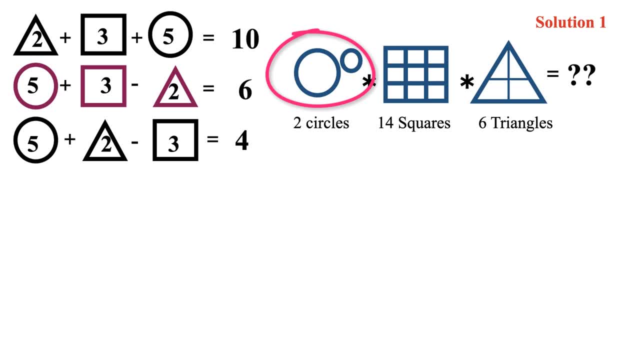 value of circle, square and triangle. substitute now 2 circles is 2 into 5, which equals to 10, since the value of each circle is 5.. 14 squares is 14 into 3, which is equal to 42, since the value of each square is 3, and 6 triangles. 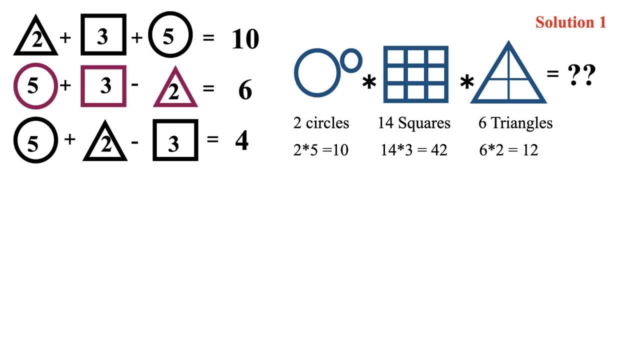 is 6 into 2, which is equal to 12, since the value of each triangle is 2. after multiplying all results, the first solution is 5040. that is, 10 into 42 into 12, which results in 5040. let's see the different. 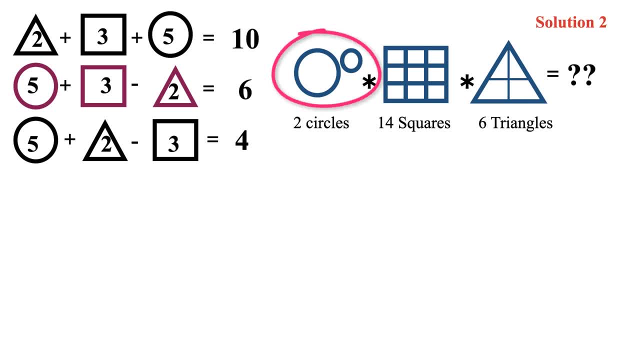 interpretation. now, if you closely look the first figure, it looks like exponential. hence it can be interpreted as 5 to the power of 5, because the value of circle is 5. after solving 5 to the power of 5, that results in 3125. thus the second solution is 3125 into 42, into 12, which 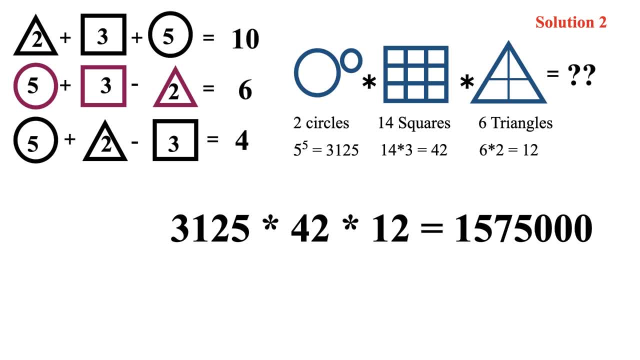 results in fifteen lakh seventy five thousand or one million five hundred and seventy five thousand. if you have figured out the solution, then you are. if you have figured out the solution, then you are. math skills is commanding. that's all for this video. please subscribe to the channel for free. 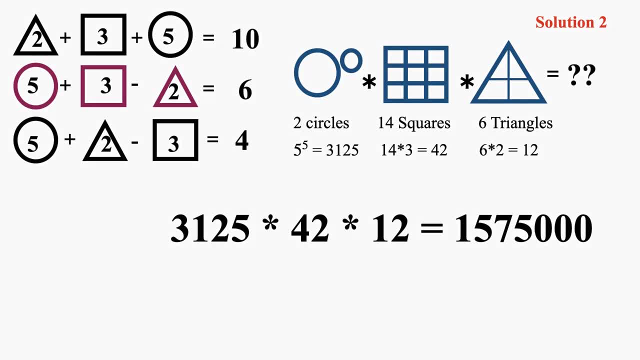 to get the newest videos watching. thanks for watching and thanks for your support. 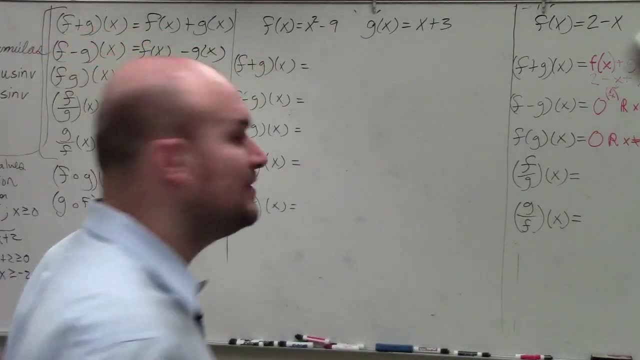 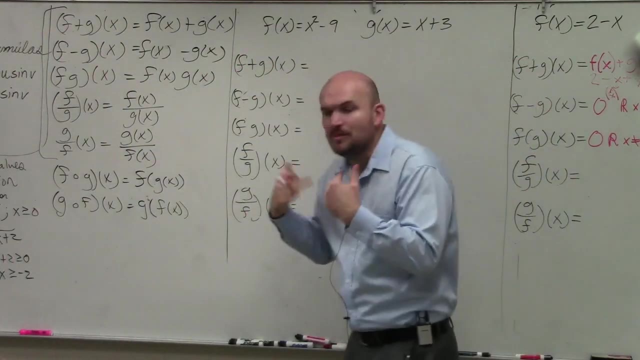 All right. So going over for these, if you're just adding them, exactly as we mentioned, f of x plus g of x is just simply f of x plus g of x. The best thing that I would recommend to do with this, ladies and gentlemen, is just take this function and then add it to that function. 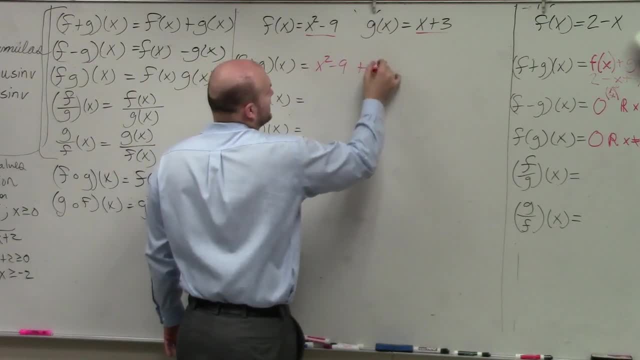 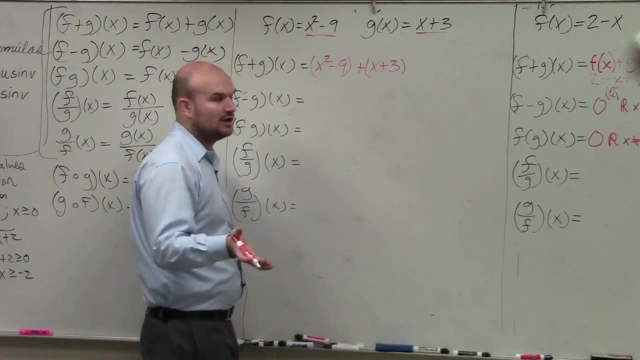 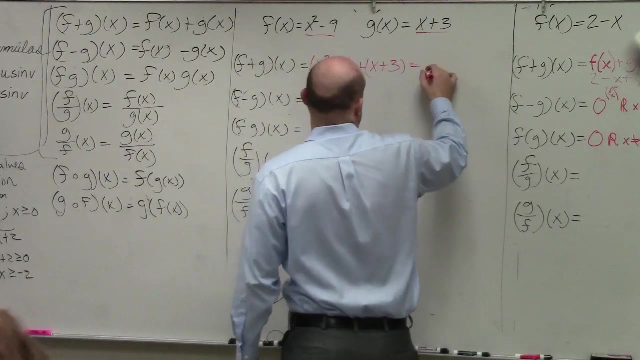 So I have x squared minus 9 plus x plus 3.. A lot of times you can put them in parentheses if you want to, but the parentheses really aren't helping us at all. The only like terms I can combine are my numbers negative 9 and 3. And that gives us negative 6.. So I have x squared plus x minus 6.. 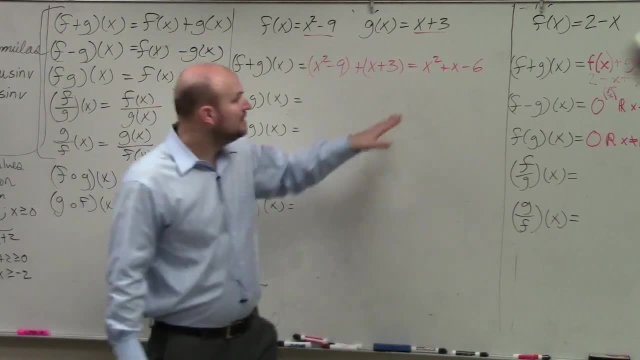 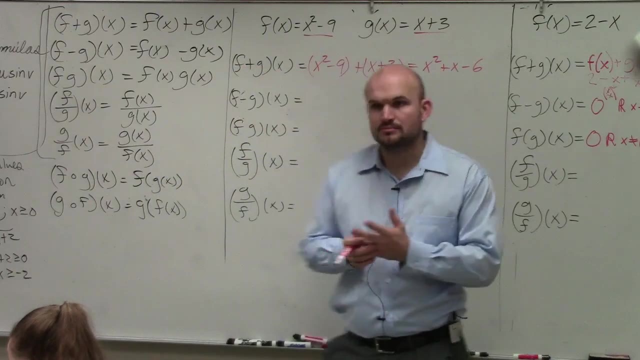 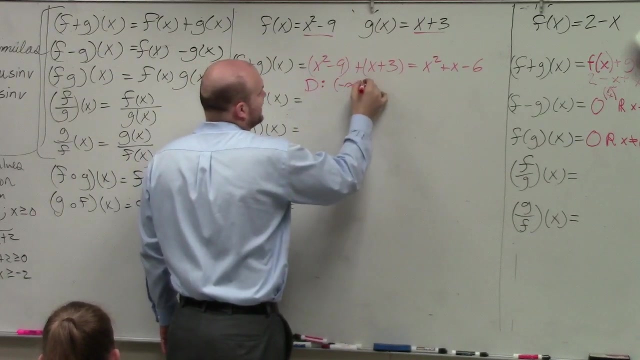 Now I asked you to find the domain for every single one of these because we've got to practice domain. Does my domain have any of my restrictions? Anything in denominator, anything under radical? Any restrictions? No, So the domain is from negative infinity to infinity. 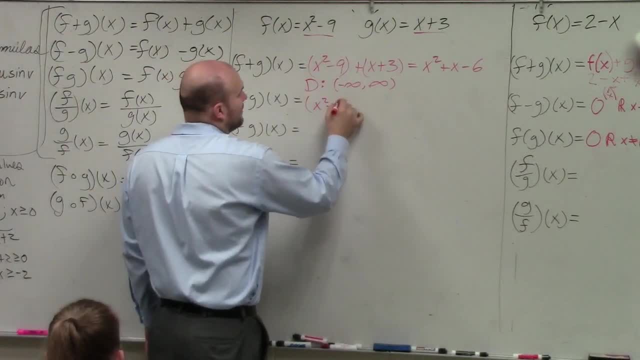 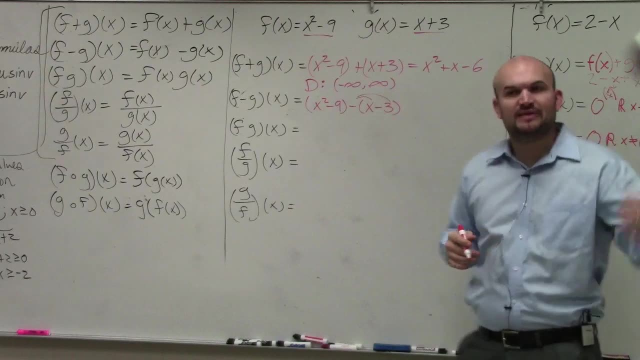 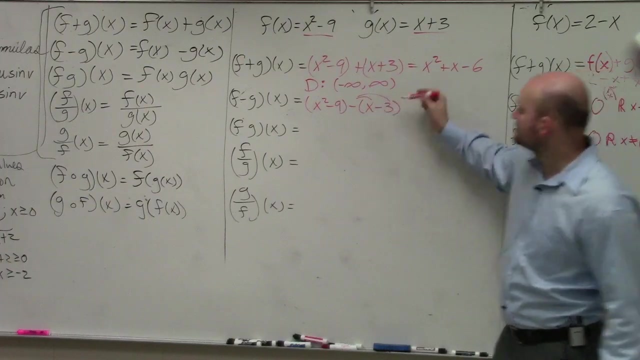 All right, Let's do f of g of x. Again the same thing. Now here I would probably recommend using parentheses, because when you use parentheses you've got to make sure you distribute that negative. So really it's a negative x and it's a positive 3, right, Oh, no, Sorry, That's a plus 3..